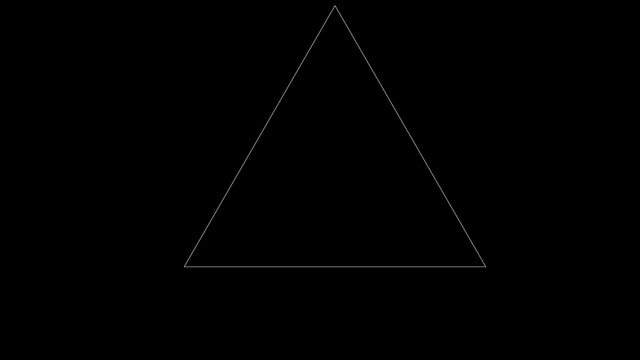 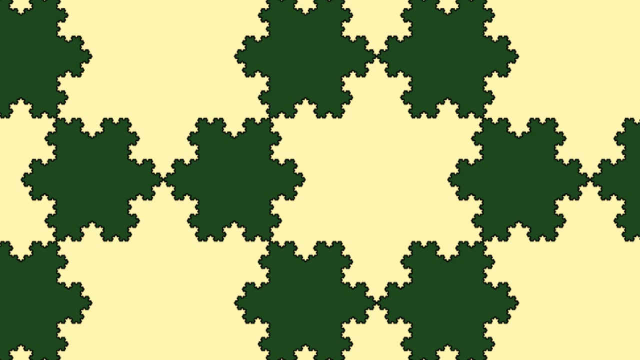 of this fractal. like I can flip a negative in the code to make the triangles point inwards, and then we get the coke anti-snowflake, which I almost think is cooler, And you can even use these snowflakes to tile the plane. I'll share some of the cool mathematical properties of the. 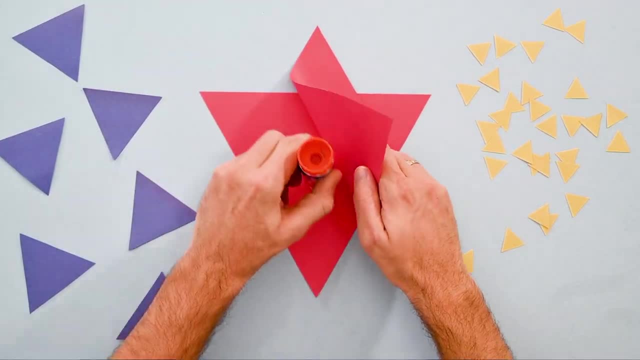 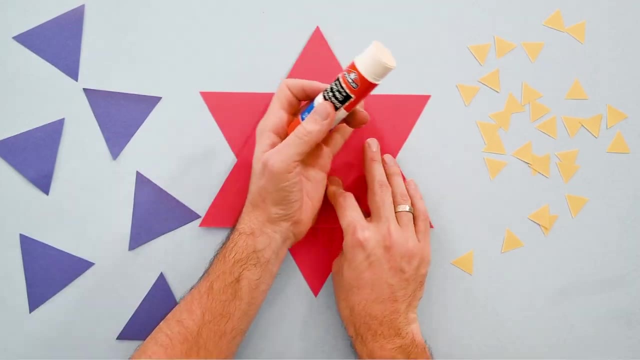 coke snowflake in a minute, but we can actually make a real world decoration out of the coke snowflake by starting with two big triangles that we glue together to be a star. I then can make six triangles whose base is one third of the size and place those six triangles so they stick. 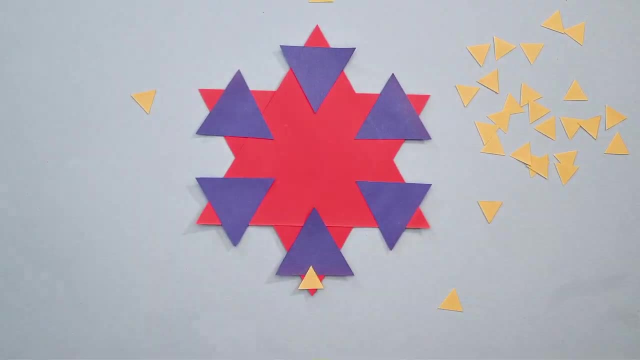 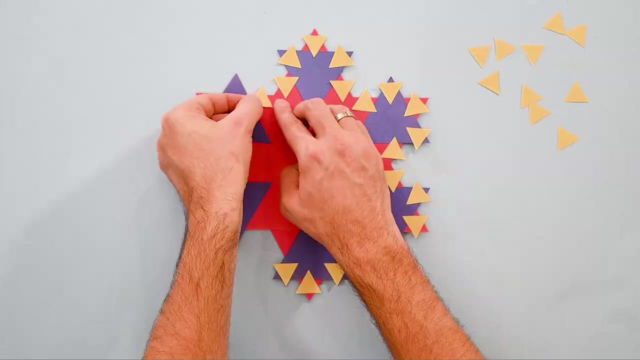 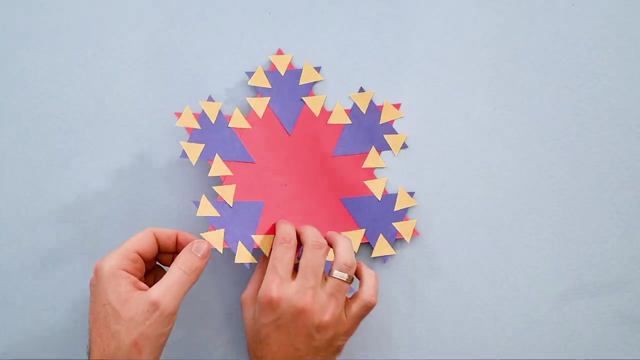 out on both sides of each point of the red star. And finally, I can use five small yellow triangles whose base is again one third of the base of the blue triangles. For each of those blue triangles, this is going to give 30 yellow ones overall And if I flip it over I get a pretty decoration that. 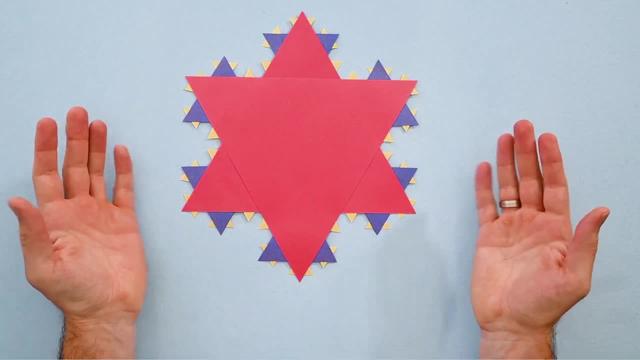 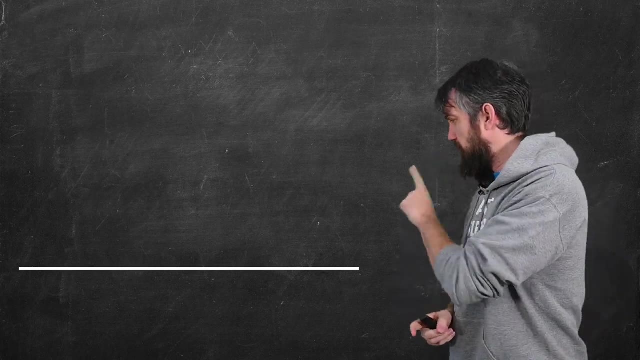 is the third iteration of the algorithm that produces the coke snowflake. Now I want to show you some really crazy mathematical properties of the coke snowflake. Suppose this is one of the segments somewhere on the snowflake and let me just say that it has length L. Then if I'm going, 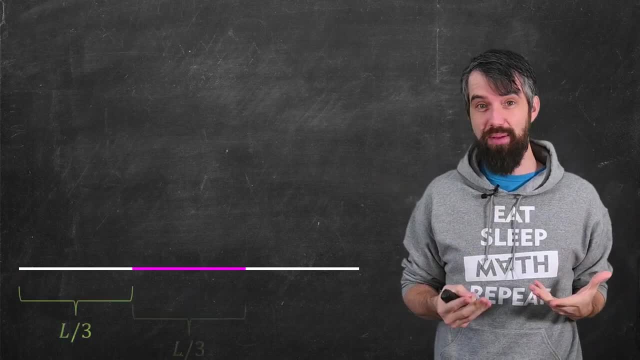 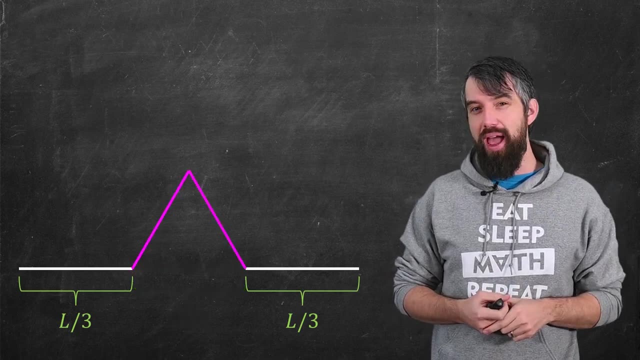 to the next iteration. I'm going to take this, divide it into three different segments, and each of these segments, now we're going to have length L divided by three. Okay, so now let me put the triangle on, And when I take the triangle on, well, the triangle is going to be the length of the. 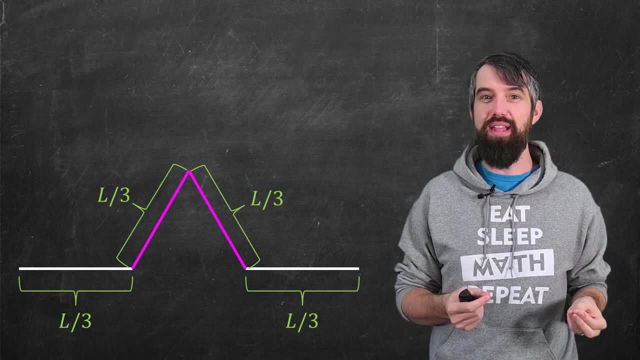 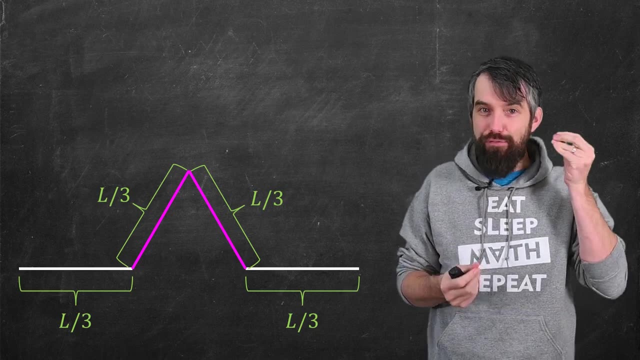 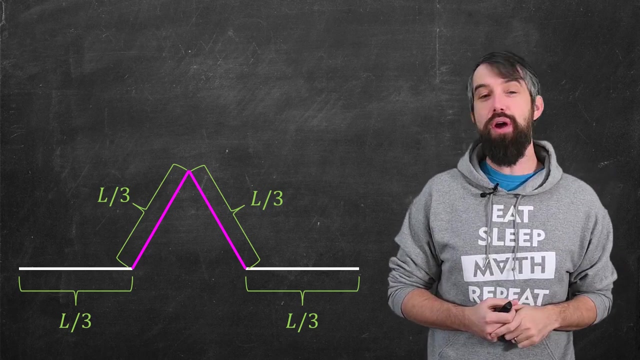 those sides, because equilateral triangles also have length L over three, And so what I've done is I've taken a length L and I've made it now a length four thirds times L. There's four of these segments that are of length L divided by three. That is, if I want to try. 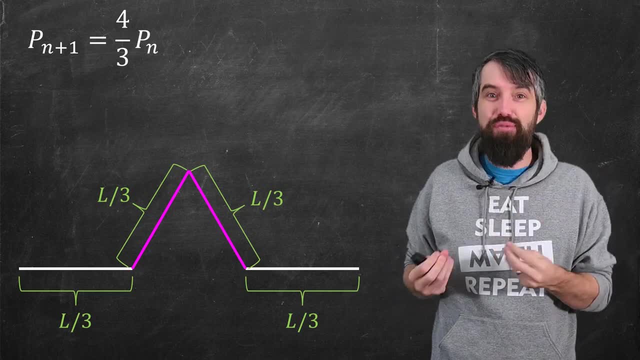 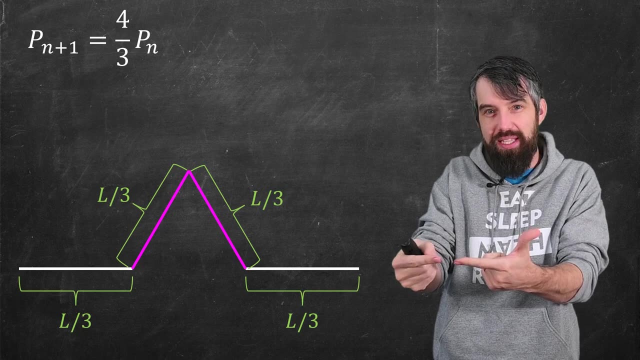 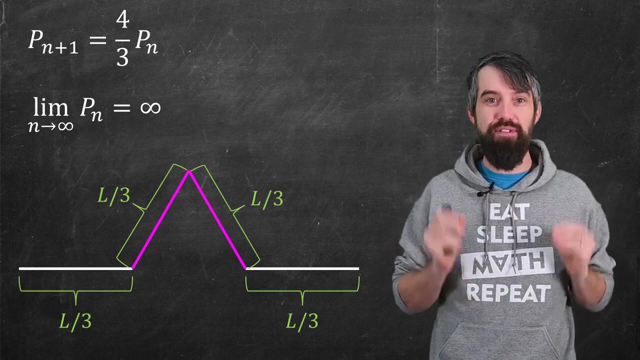 to describe what the perimeter of the coke snowflake is going to be. well then, it's just four thirds times what the perimeter of the previous iteration was. Take the limit, as n goes to infinity and this is going to diverge, So the perimeter of our snowflake diverges to infinity. 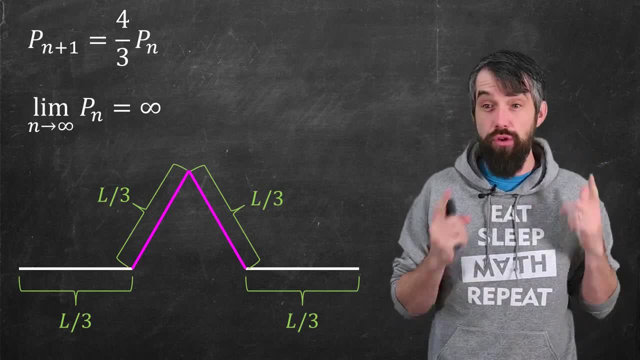 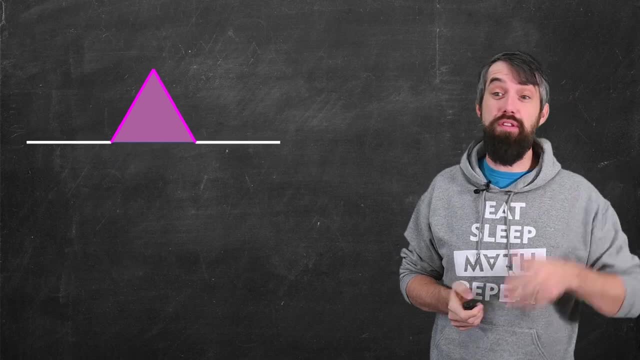 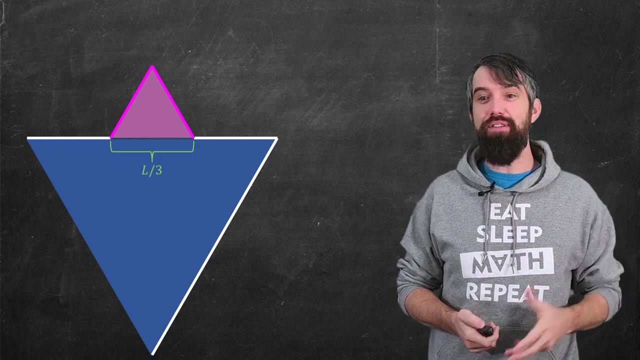 But what about the area? So same sort of thing. I've added a new triangle and I want to say: well, what's the area of this new triangle that I've added? Now, this line segment was part of some previous triangle, somewhere else on the snowflake, And because it had originally a base, 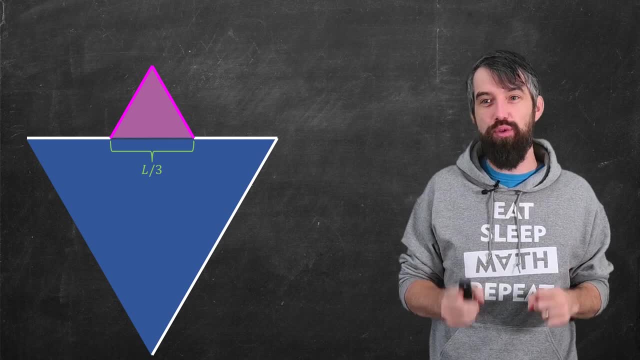 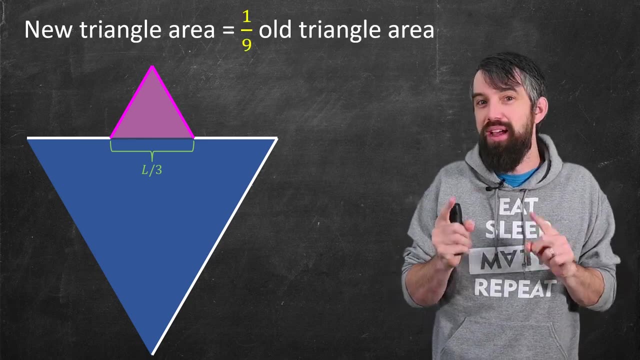 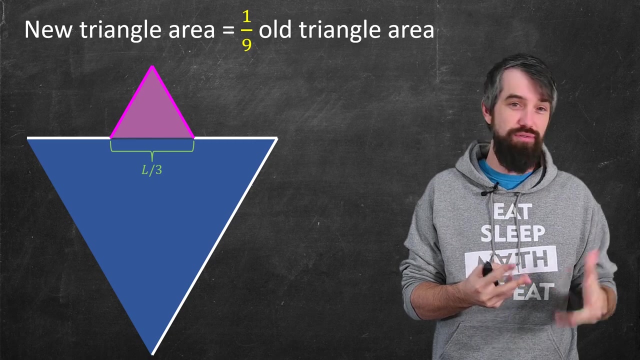 of L, but now the new one is a length L divided by three: the base to the area. the one third gets squared and becomes one ninth the size of the original triangle. So every time you add a new triangle in your new iteration of constructing this crazy. 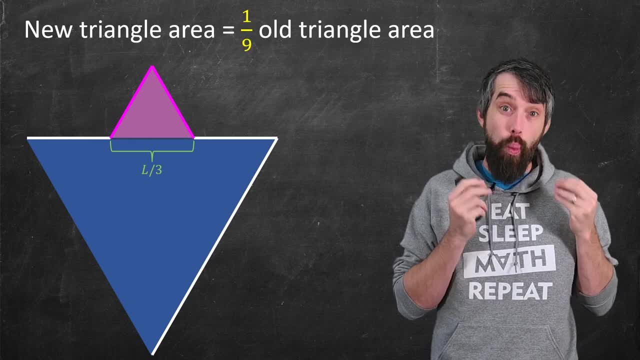 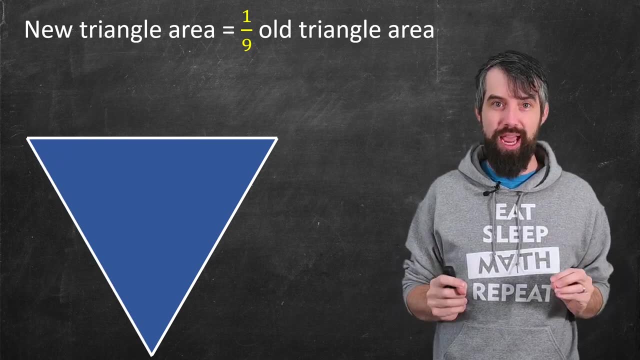 snowflake. what you're really doing is adding triangles of area one ninth, the previous step, Okay, but how many are there going to be? Well, let's go back actually to the very original step, where you just start with the triangle itself, That is, it's got all three sides. Maybe I'll say it's a. 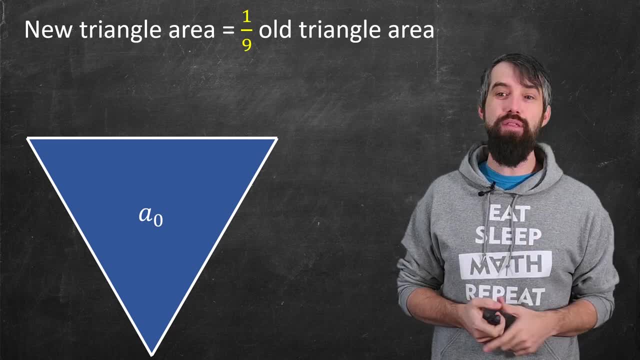 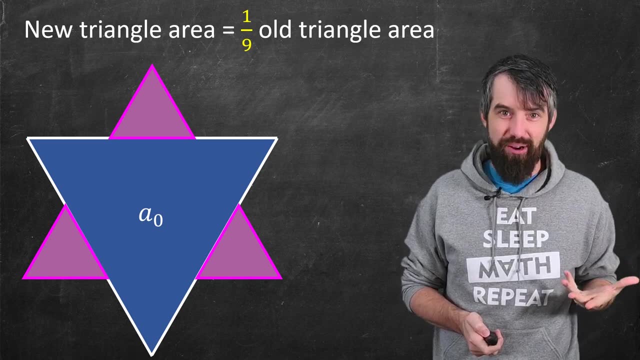 triangle of area one, and then I'm going to add, well, three triangles onto it, And here each of those triangles is one ninth of the original area. So the original area is A-naught. Then I'm going to have A-naught divided by nine for each of these triangles Going from the first. 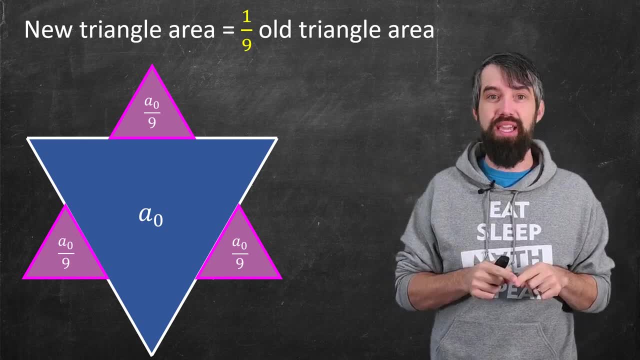 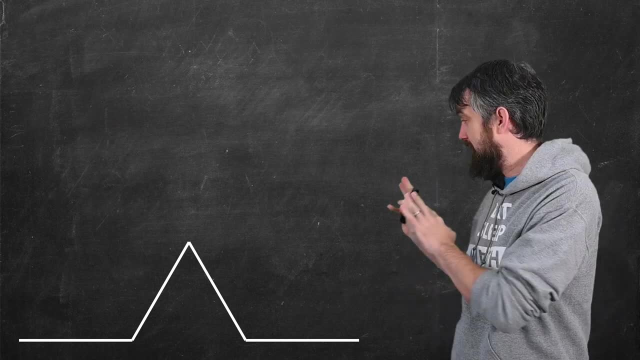 to the second step was quite special because the very first step just begins with a triangle that's sort of closed. But something different happens for all subsequent steps, That is, let me just imagine I have a segment somewhere in my snowflake that looks like this: 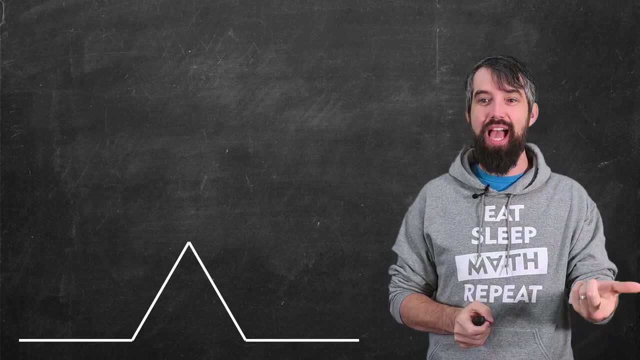 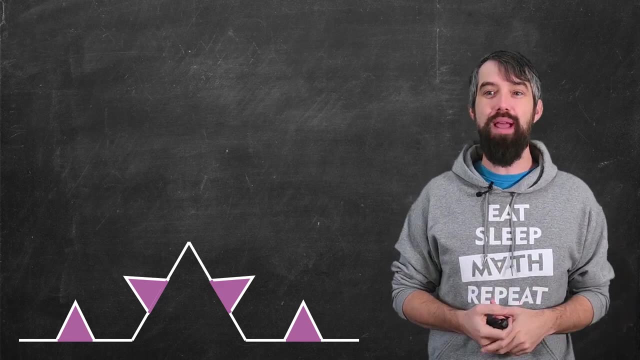 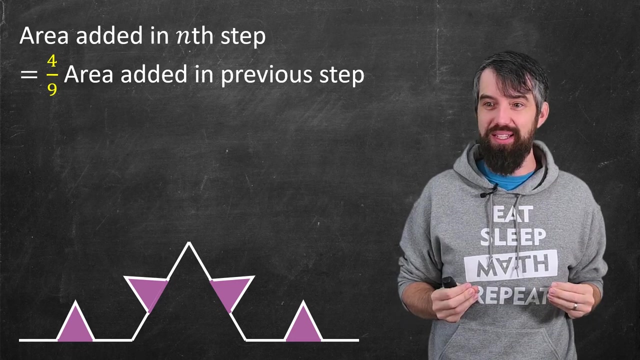 There's four segments and so if I go to the next iteration I get four different added triangles, each of those one ninth the area of the previous step. So really what I'm saying is that the area added in the ninth step is four ninths the area from the previous step, The one ninth because 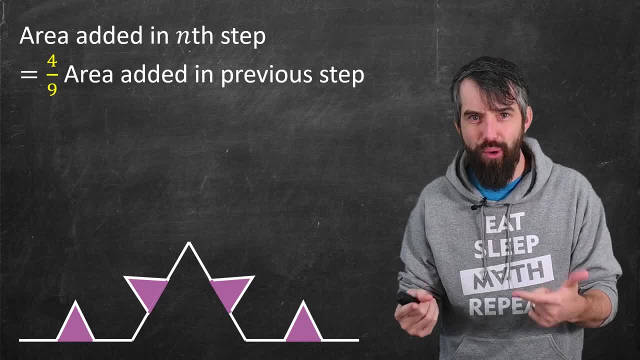 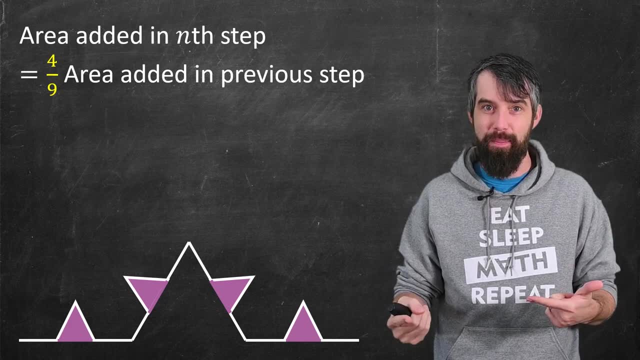 all of my triangles are one ninth as large. and then the four is because, for whatever triangle I added in the previous step, I'm now adding four new triangles in the next step. Okay, so let's put that back together and try to figure out what the area is. Okay, it's a big, long, messy expression, So what's? 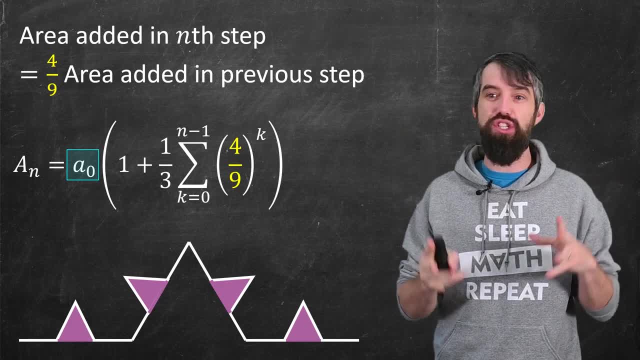 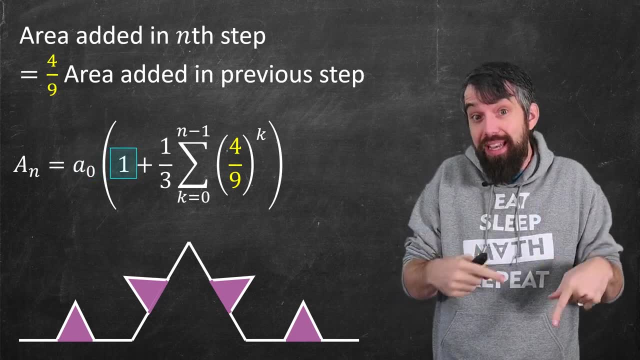 going on Out the front is the A-naught. This is the area of your original triangle. just some fixed number, Maybe it's just one? Then I multiply by one to say: well, I have that first triangle. but then the next thing I'm going to be doing was adding three triangles of length, one over nine. That was. 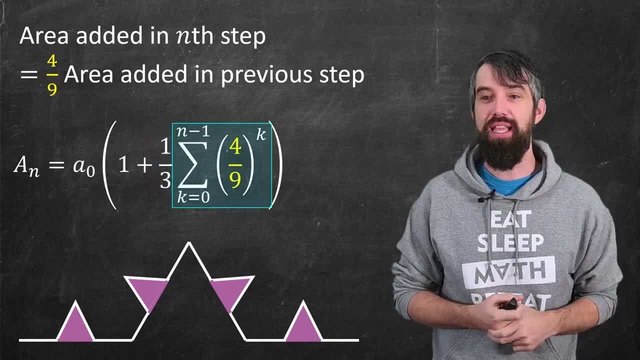 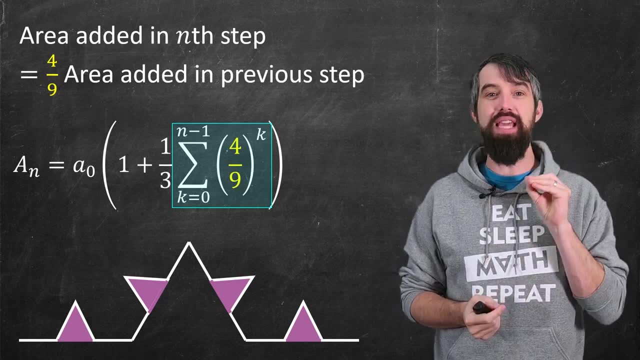 why I have this one third stuck out the front. Everything else in this infinite sum says: for every iteration after that, k zero, all the way up to n minus one, I'm going to be adding four ninths the area of the previous step, every single time. Now we can use the power of calculus. This: 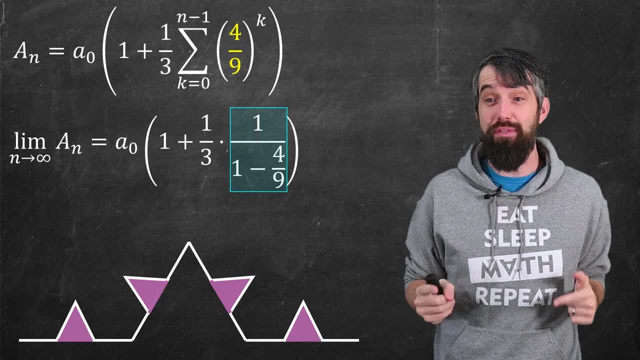 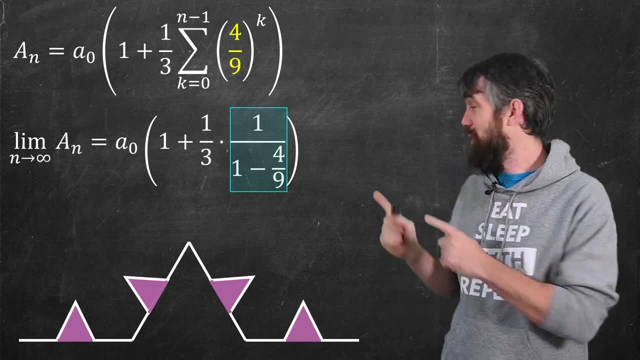 is a geometric series, So if I want to take the limit as n goes to infinity, I know how to replace the sum of r to the power of k. It's one over one minus r, So I can plug that in. This is just some. 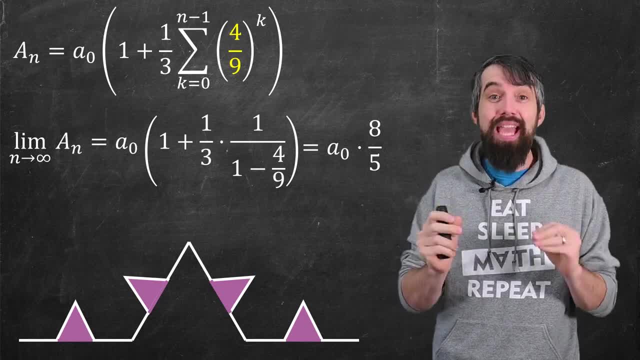 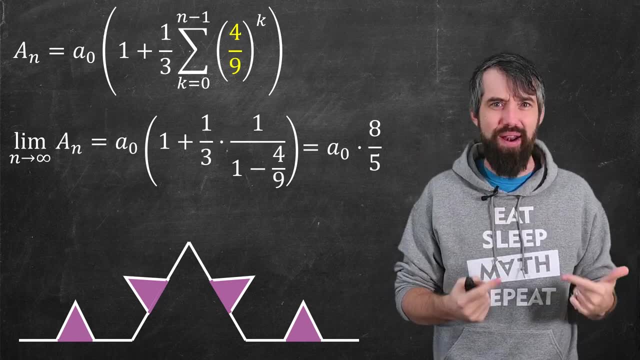 number And what do I get? I get A-naught times eight fifths. The area is finite. It's just eight fifths the original area. So what we've got in here is the area of the original triangle. So what we've got. 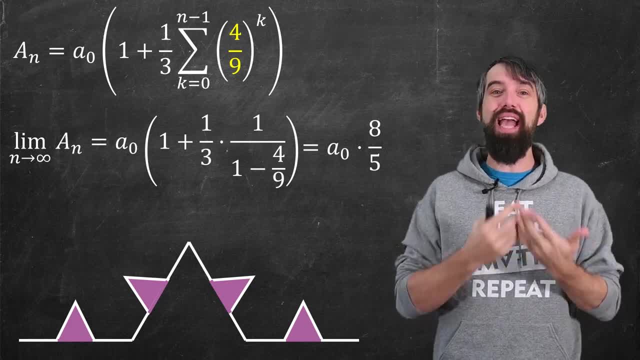 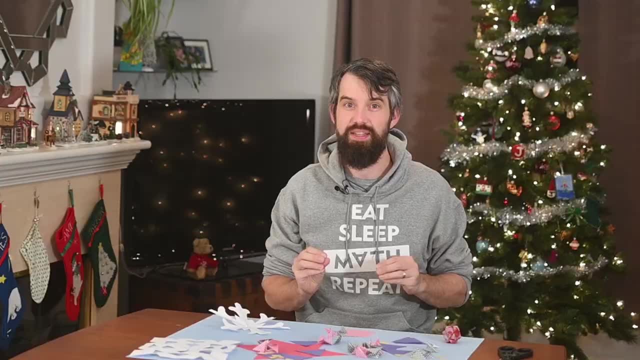 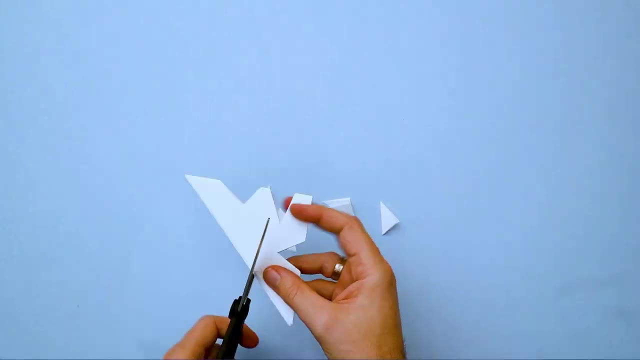 is a finite interior area, nevertheless an infinite perimeter. Fractals are just so cool. Next up, let's talk about the symmetries of snowflakes. I'll start simple with a square, folding it in half into a triangle three times, and then I'm going to cut some random shapes. 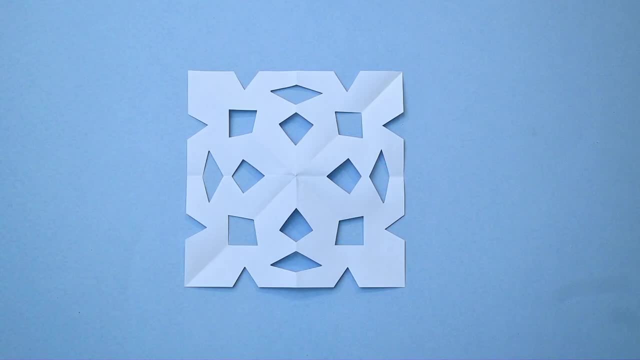 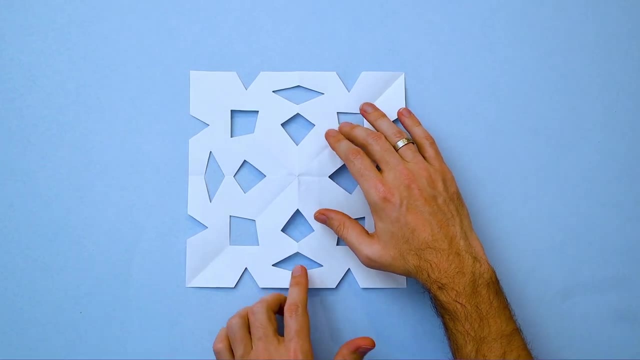 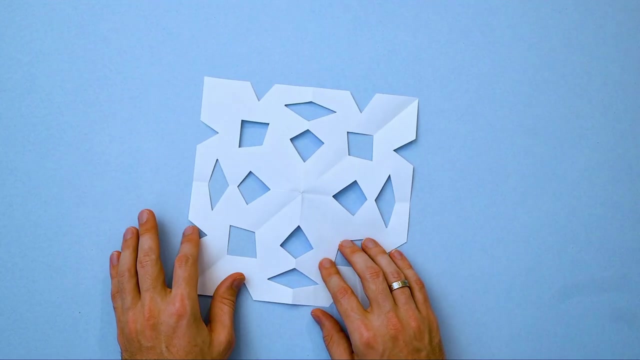 When I unfold it, I get a pretty snowflake. What I'd really like to do is think about the symmetries of this object that I've created. One of the first things I notice is that if I rotate it by 90, 180 degrees, 270 degrees or 360 degrees, it looks exactly the same every way that I do that. 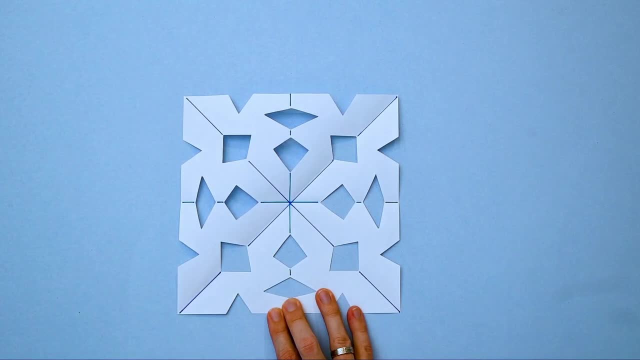 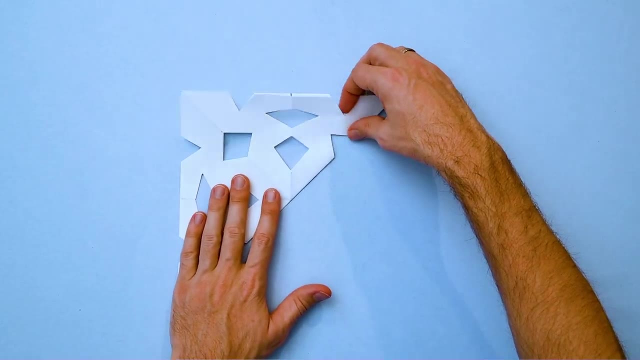 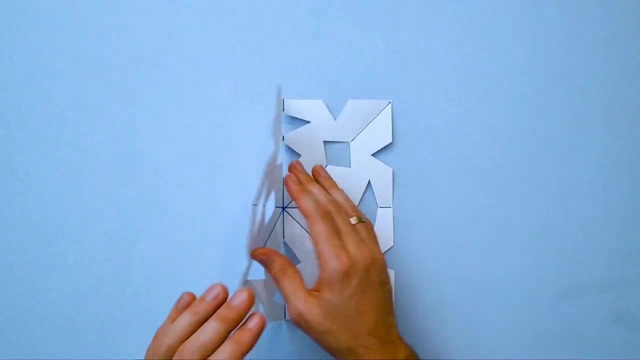 In addition, if I draw these four lines, I also have four different axes where I can reflect over. For example, I can reflect over this diagonal line and I get precisely the same shape. Or I can flip it over the y-axis and I get precisely the same shape. And so this snowflake that began as a 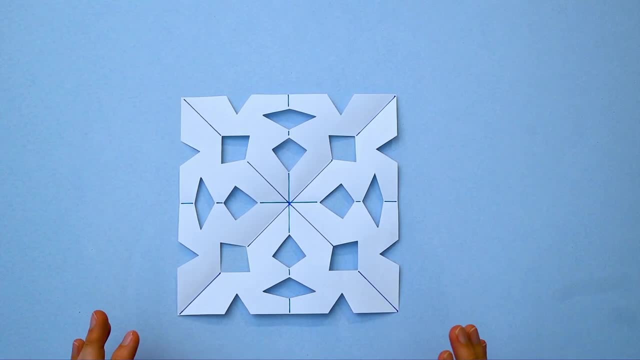 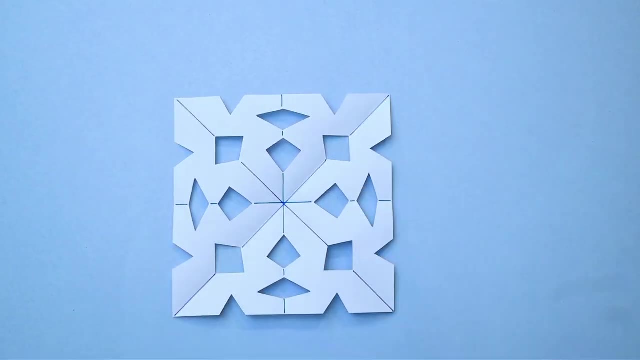 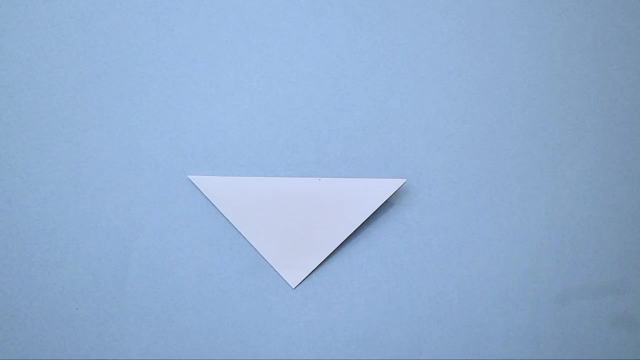 square actually has eight different types of symmetries: The four different rotations by 90 degrees and these four different axes of reflection, eight in total. Now, real world snowflakes like this one usually actually have six major points, And so let's instead fold our square. 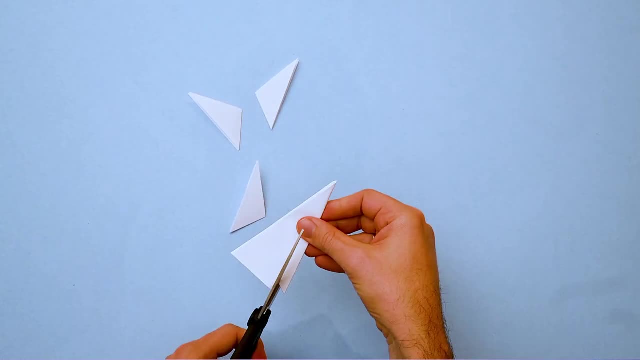 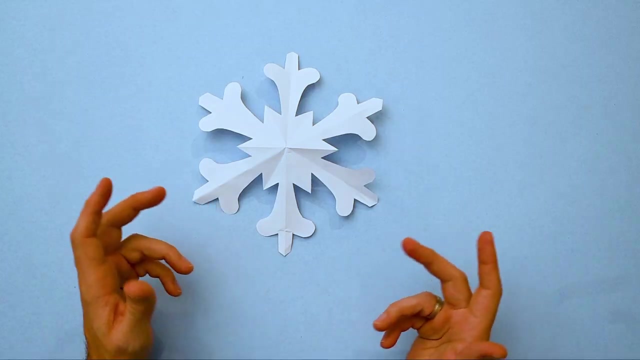 cut it in a way that makes a hexagon and then I'll cut away from that hexagon whatever pattern you like, where we have a really pretty paper snowflake built out of a hexagon. And when I unfold it I see that there are six different points. They're all roughly symmetric. 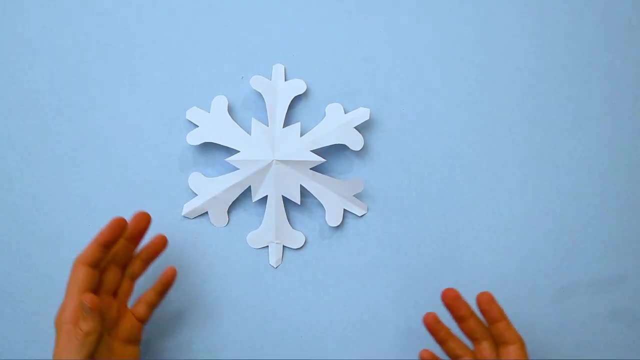 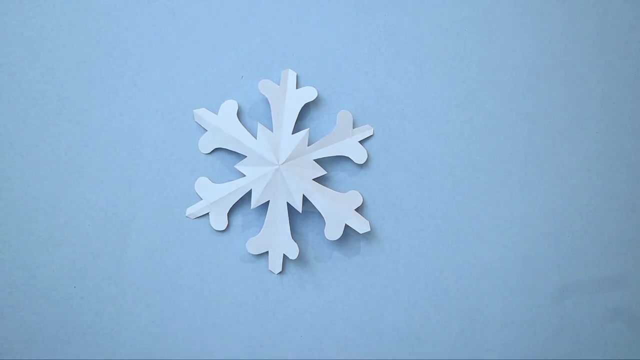 up to my ability to fold and cut nicely. Taking 360 degrees and dividing it by six, that gives me 60 degrees, And if I do a 60 degree rotation I end up exactly where I started: Six different axes I could reflect around. So, for example, if I rotate over this line here, I'm going to get 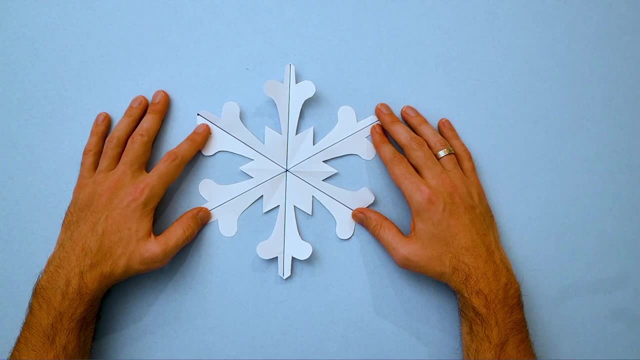 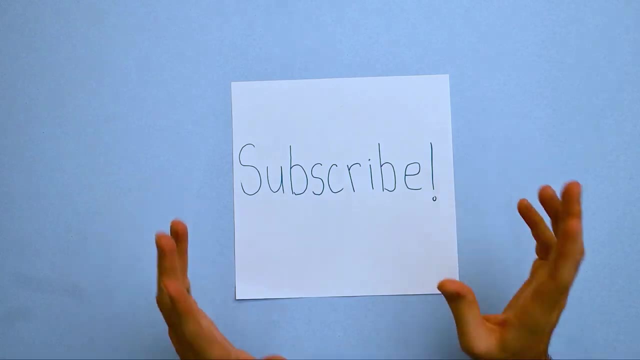 a precisely symmetrical object. The group of symmetries here is now called D6, the dihedral group with six points, And if I rotate it over the hexagon it's going to be exactly the same. So six rotations and six reflections. Let's go back to the square, And I've made this not symmetrical. 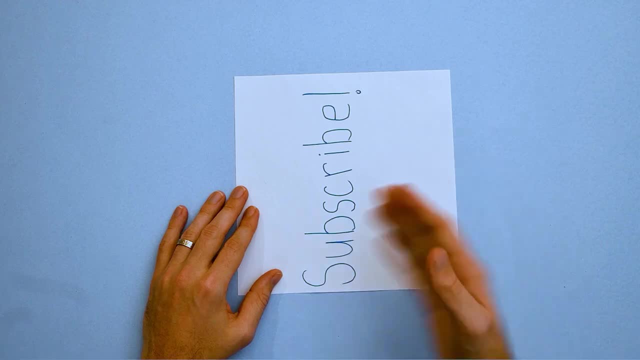 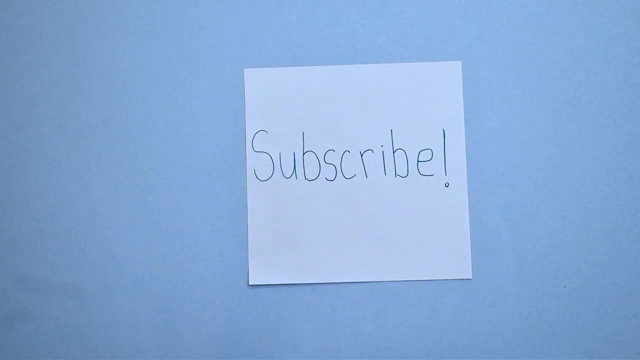 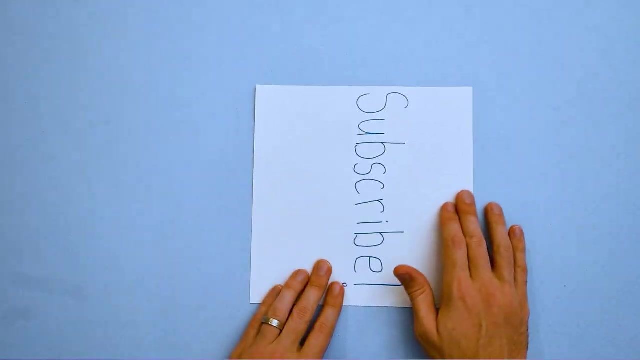 as in: if I rotate by 90 degrees or pi over two. well, it looks different. the subscribe is going this way, But this is helpful for us to illustrate various properties of the symmetries of squares in general. For example, if I rotate 90 degrees, 90 degrees, 90 degrees and then 90 degrees, 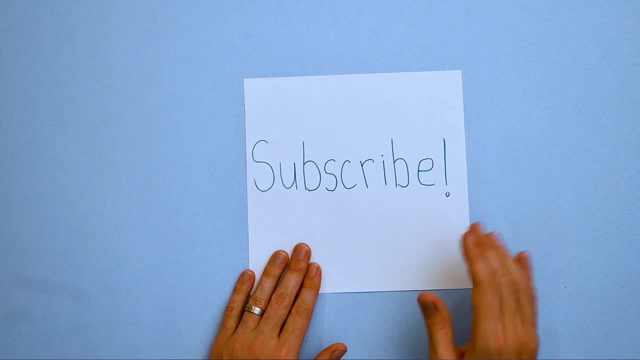 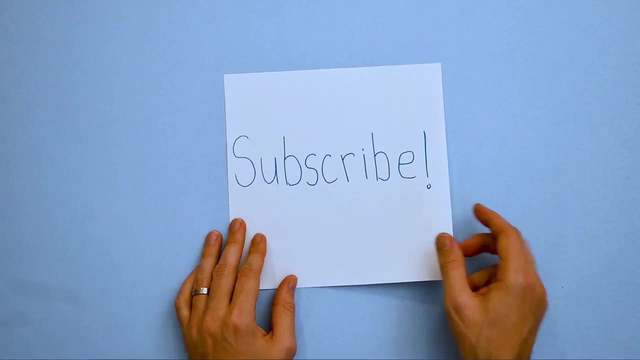 again, I get to 360 degrees. I'm back where I started and it reads completely Proprily: Similarly, if I reflect around the axis and then reflect around the axis again, I get back to where I started. So two reflections along the same axis lead to the same result. But then I can have some slightly funkier things. For example, suppose I rotate by 90 degrees and then I was to flip over the x axis, leaving this location. However, what if I went in the other order? Suppose I was to reflect over the x axis and then rotate. 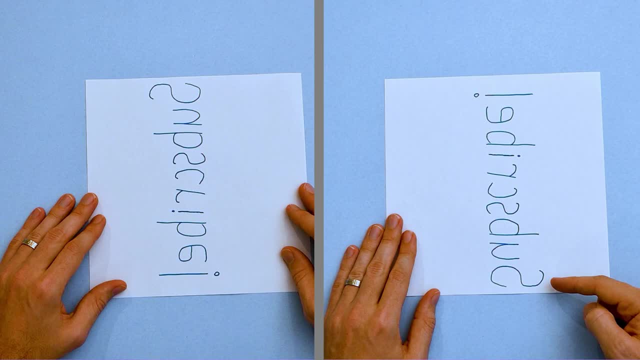 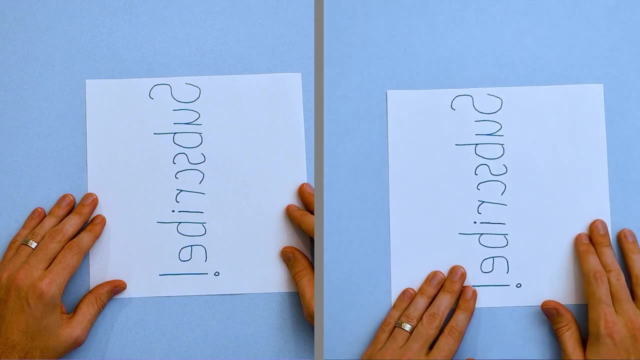 by 90 degrees. Well, this is not what I had just seen before. this has got the exclamation point up at the top, But if I then rotate a second time and a third time, I'm in precisely the scenario that I was just in, Which is to say that if I rotate and then flip, I've gotten the same result. 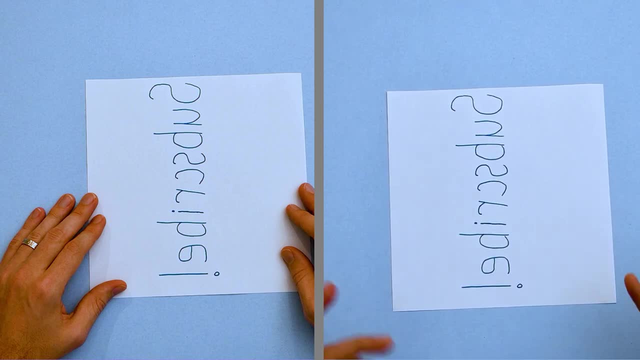 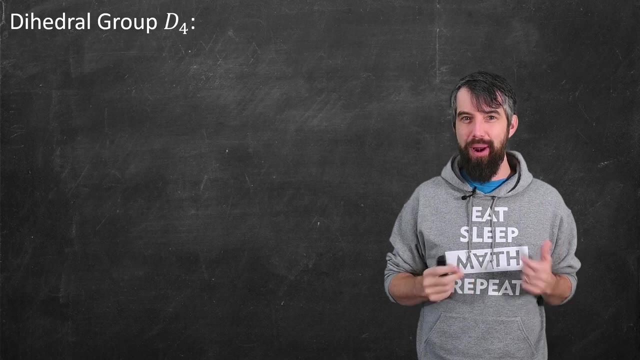 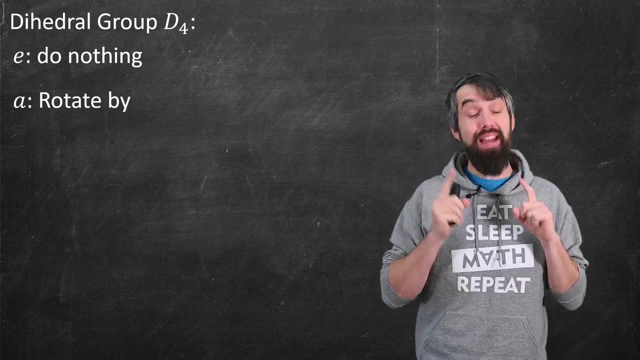 as if I flip and then rotate three times. So what exactly is going on here? Let me be a bit more specific about what's going on with this dihedral group. Well, what I'm going to do is define e to be the thing that just does nothing, just leaves your object exactly where it is. I'm going to define a. 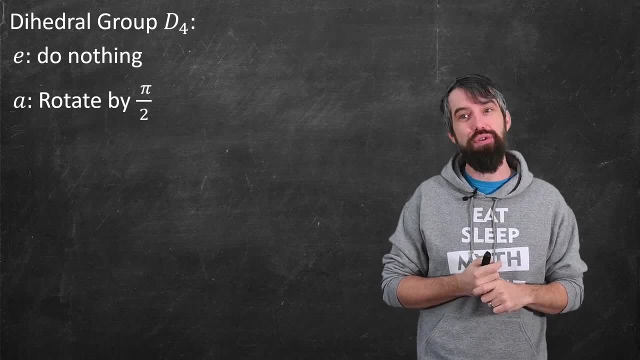 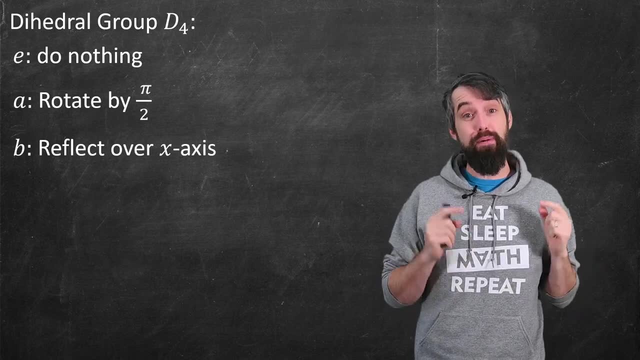 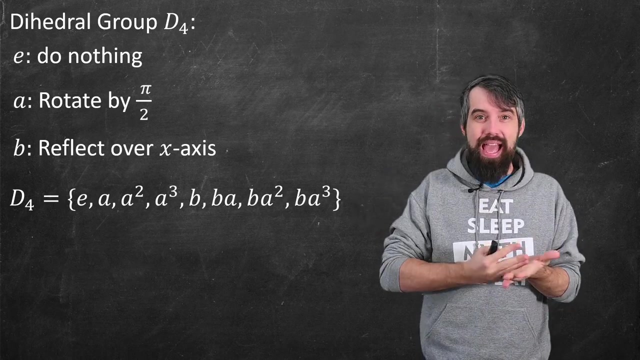 to be a rotation by pi over two. specifically, I'll do a counterclockwise rotation and then for b, I'm going to denote that reflecting over the x-axis. So my preferred way to write down the dihedral group is actually the following. I like to list it as eight elements: e, a, a sub and b. 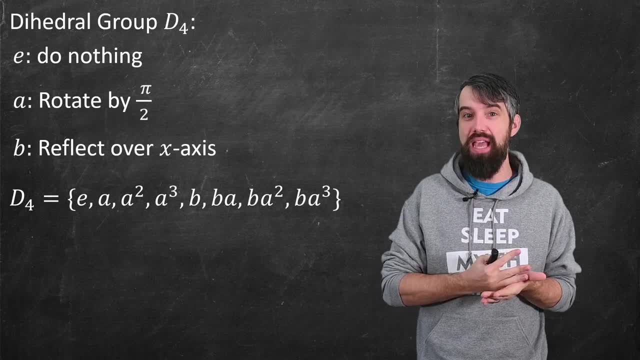 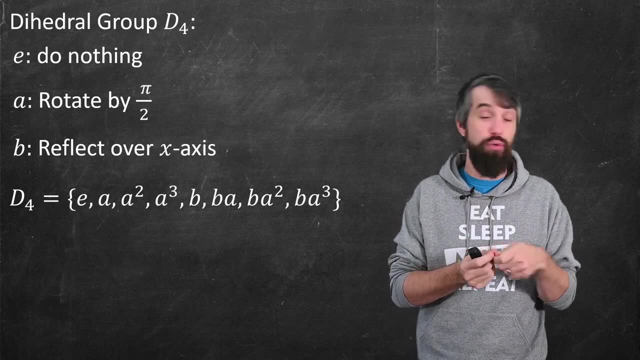 So b squared, a cubed, b, b a, b a squared and b a cubed. What I'm basically doing is listing down all the ways that I can mash together, doing some combination of the rotations, Like, for example, rotation by pi. I don't. 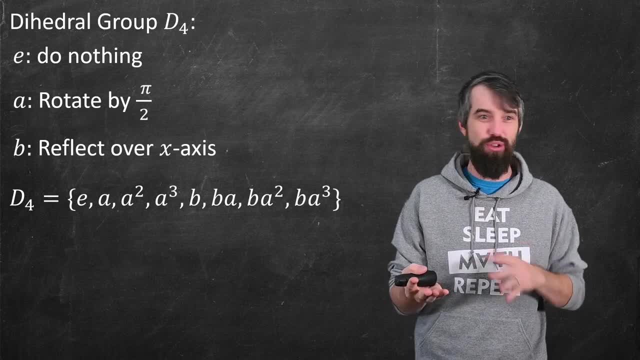 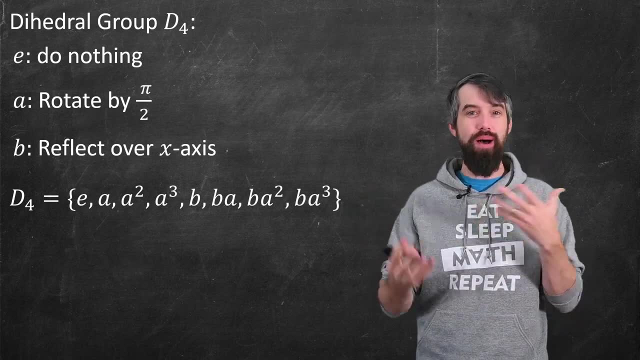 need to give it a new name. It's just a squared, because you rotate by pi over two, and then pi over two again, and you've rotated by pi. So you then might say: well, hold on, you haven't written down every possible way. I could combine an a and combine a- b. There might be a whole bunch of other ones, but 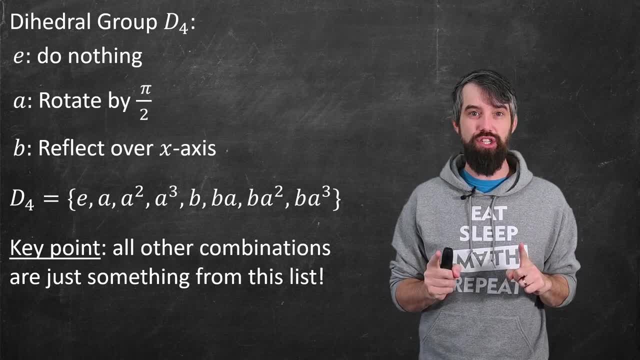 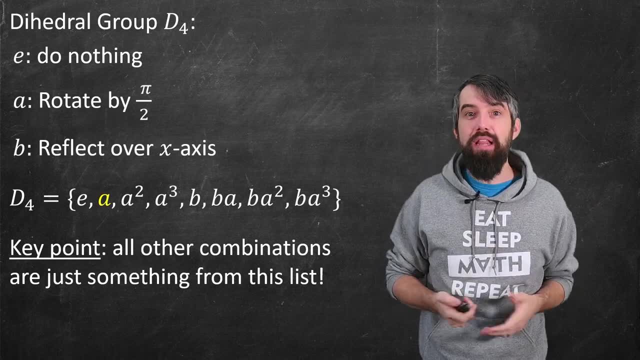 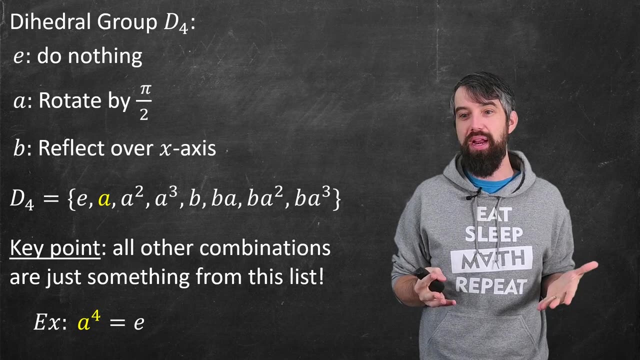 the big idea here is that all other combinations are actually already on this list. For example, let's take the point a. I've got a, a squared, a cubed. What about a to the fourth? Well, a to the fourth is just rotating 90, 90, 90, 90 as 360 degrees, or two pi radians. 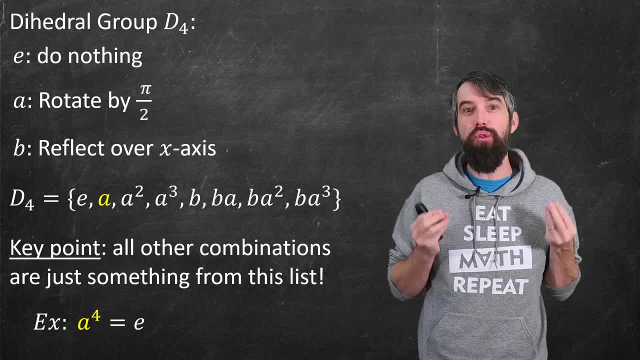 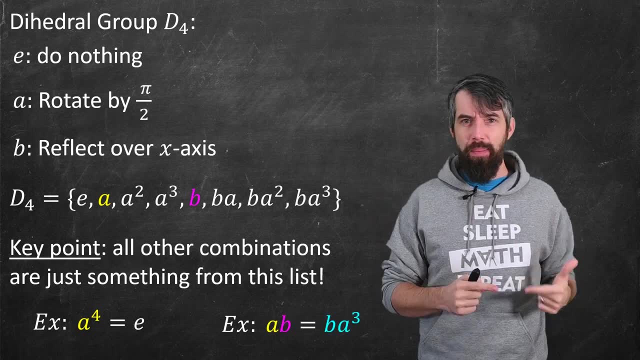 That's just getting right back to the thing that does nothing, which we called e. So a to the fourth is on this list. it's just not written that way. It's written as e Or for a more complicated one, as we saw earlier, it's called a. 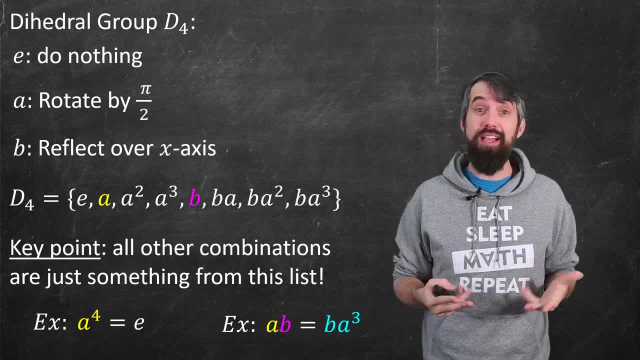 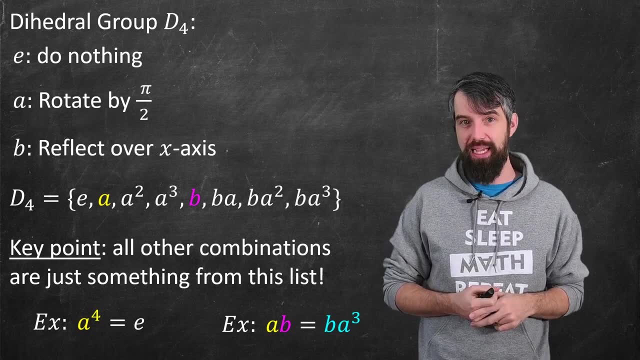 If you decide to rotate first and then reflect, this is the same thing as reflecting first and then rotating three times. a b is equal to b a cubed- another thing that's already on my list. It's worthwhile sitting down and trying to play with these combinations and convincing yourself. 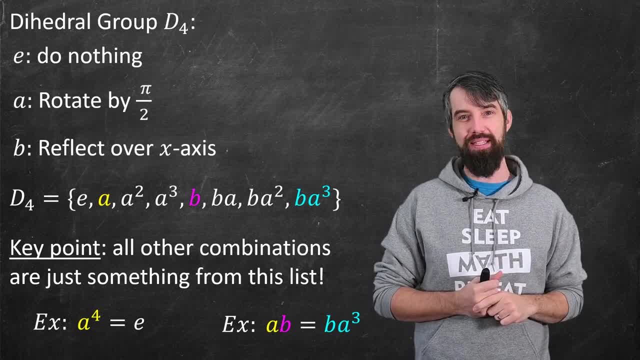 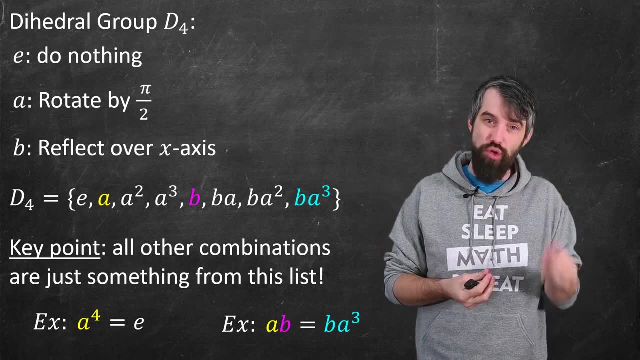 that this list of eight elements is all the possible ways. In math speak, what we say is we have a binary operation, which means if I take any two elements from the set and combine them like do one then do the other, then the result of that is something that is in the set. It is. 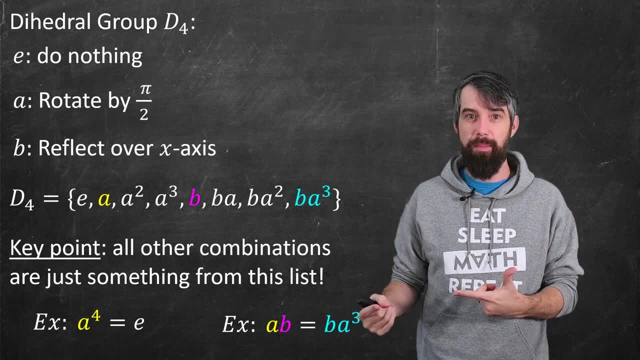 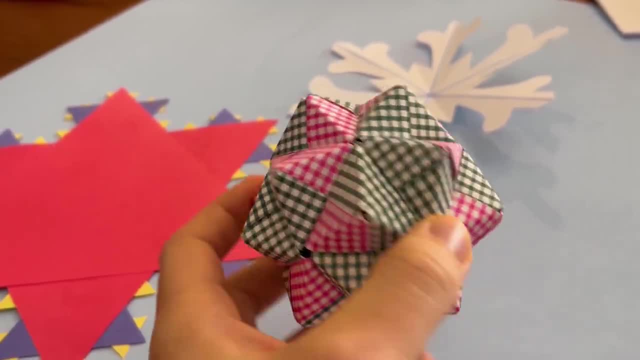 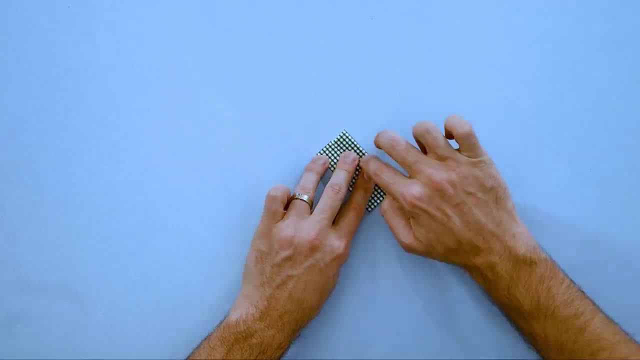 so-called closed under this binary operation. The final decoration I want to show you is how we can make an origami stellated dodecahedron, which are just lots of fun. I'm going to start with a little square piece that I fold in half and then fold each half in half again. I bend down. 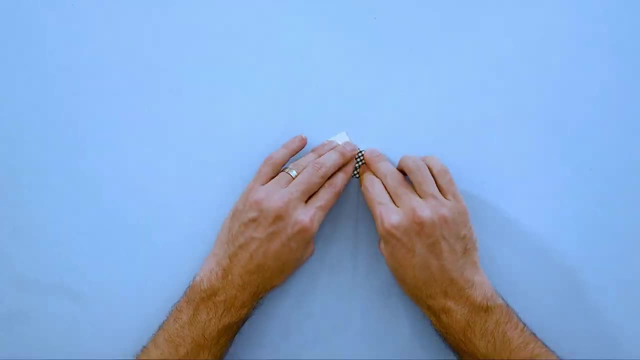 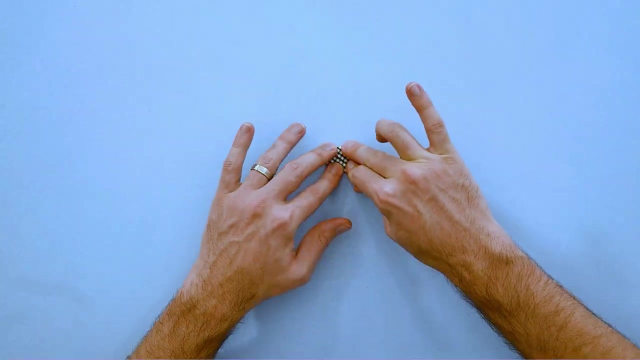 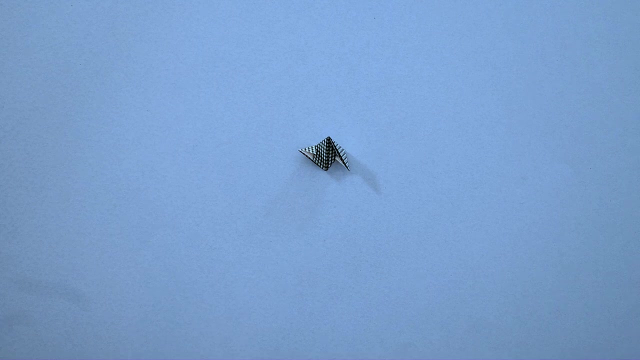 the top right corner to the left side, rotate it and bend the other corner to the side. Then I'm going to fold the top triangle down to the midline, rotate and fold the other triangle down to the middle. This basic shape can be used to make all sorts of cool things, and this dodecahedron. 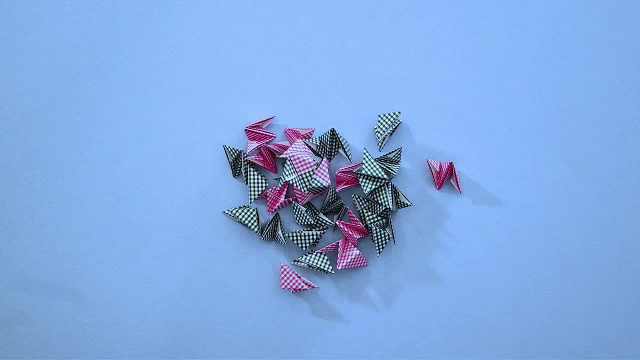 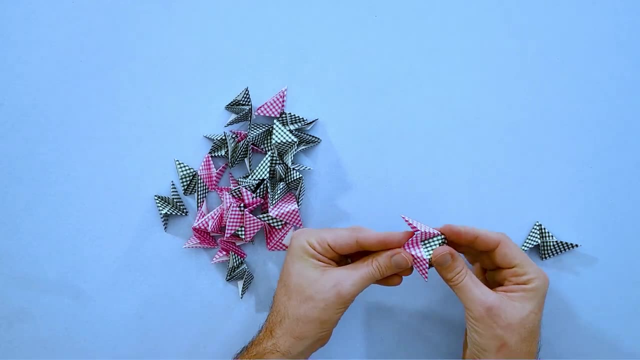 requires 30 of them. Now it's time to assemble. You can take the corner of one of the pieces and stick them into the folds of the other, like this: The immediate goal is to make lots of little pyramids with three separate corners from three separate pieces all sticking into the folds of. 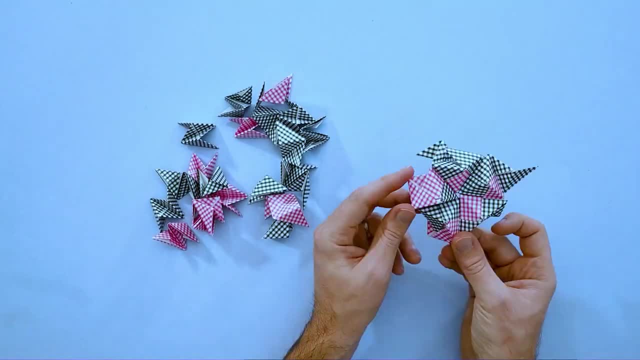 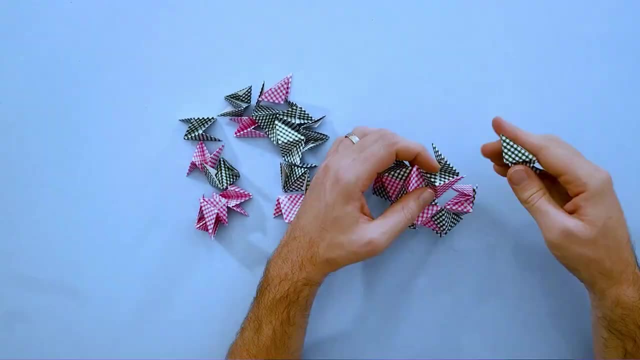 each other And we keep doing this with the basic goal that around one of the central holes there will be five mountain peaks. I usually screw this up and sometimes the patterns will have four peaks or six peaks, which give other interesting objects, but we are aiming for five in our 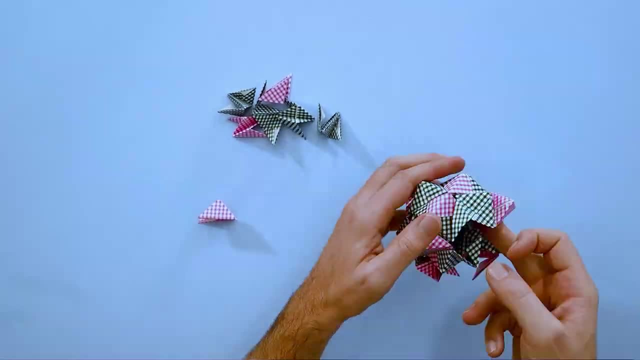 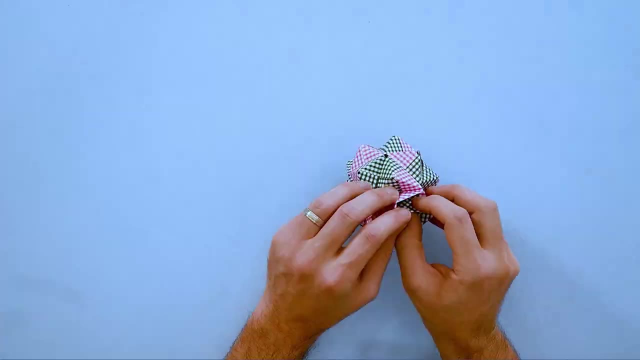 dodecahedron. Anyway, after you get your first five peaks around one of these holes, you keep going like this and we'll eventually close it off, And the last couple are a bit finicky. but there we are. We finally have our beautiful dodecahedron Now, if you really want to master, 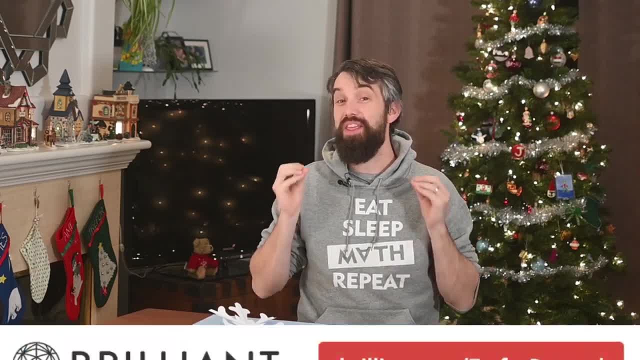 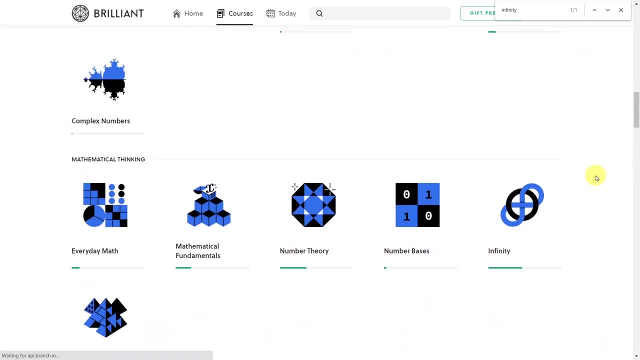 mathematics and not just make pretty math decorations all day, then I would highly recommend the sponsor of today's video, which is brilliantorg. Brilliant has thousands of lessons on mathematics, science and computer science, but what I really wanted to show you today, 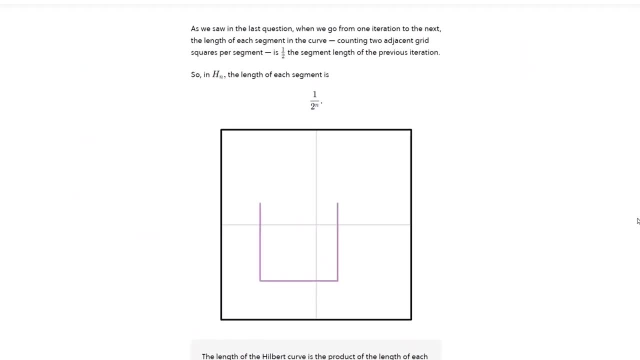 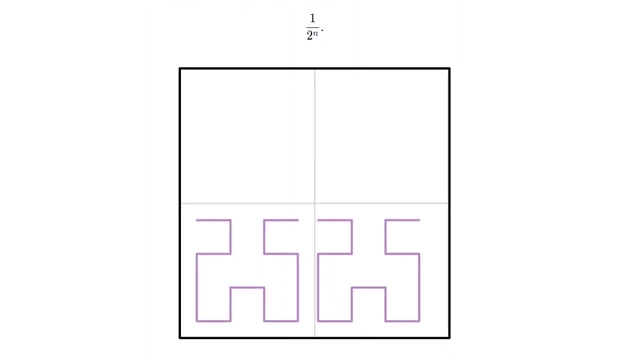 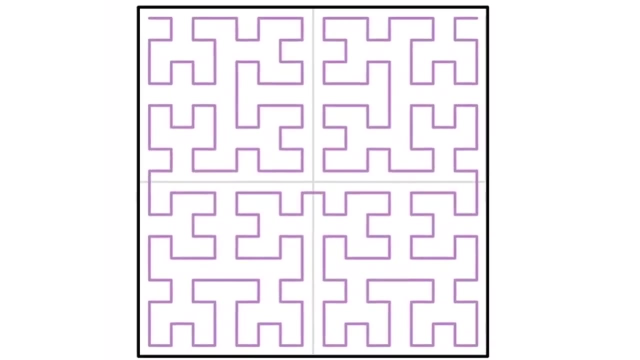 is this lesson in their infinity course on another really cool fractal called the Hilbert curve? This so-called space filling curve has the remarkable property that the one-dimensional curve is eventually going to be filling up an entire two-dimensional space. Cool right. 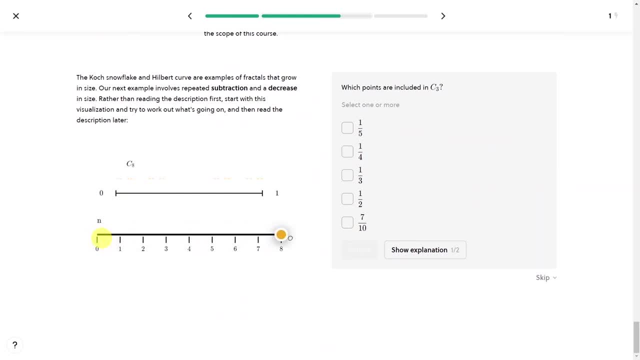 But what I really like about Brilliant is just how interactive their lessons are, Whether it's playing with the graphics, testing my knowledge or checking out the explanations. if I don't quite understand a question, yet, Brilliant puts you in the driver's seat As a math professor. 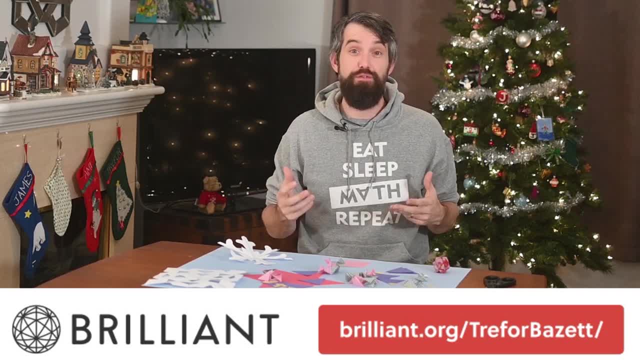 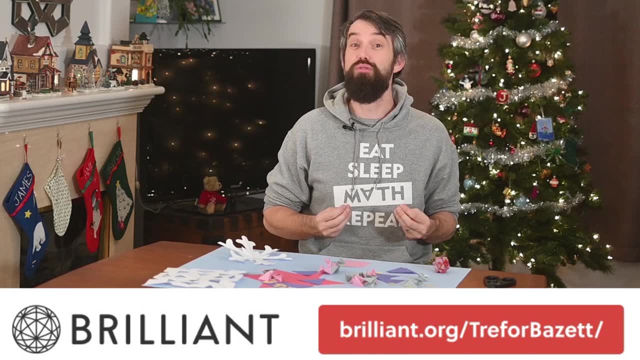 I know that this kind of active learning approach is highly effective for both learning mathematics and becoming a better problem solver, and that's why I'm so proud to be sponsored by Brilliant. So go to brilliantorg. slash Trevor Bazit or click the link down in the description to sign. 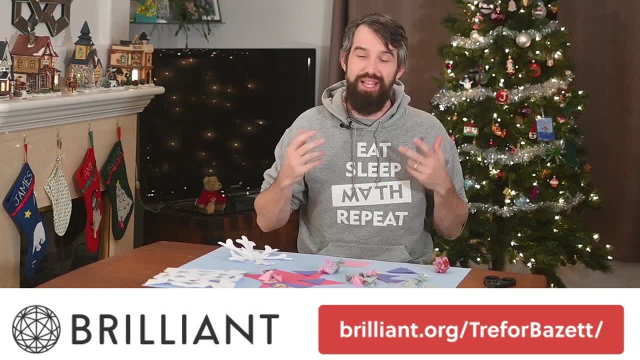 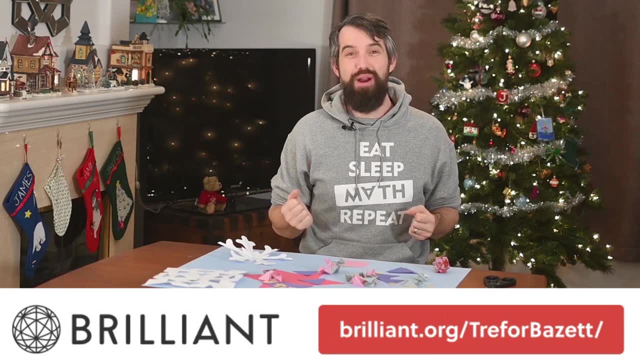 up for free. Also, the first 200 people to click that link are going to get an extra 20% off their annual premium subscription. With that said, if you have any cool math crafts, I'd love to see them down in the comments below. Give the video a like and we'll do some more math in the next video.